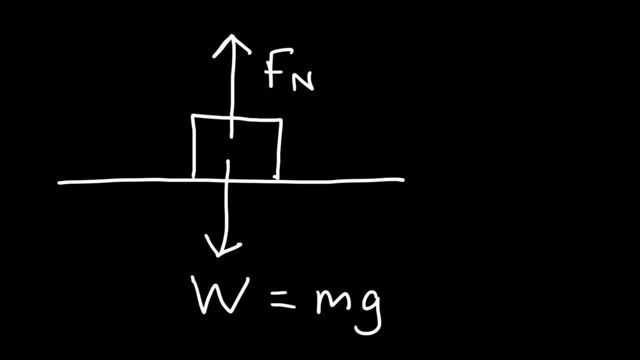 known as the normal force. So the normal force is always a force that is exerted by a surface in response to another force, So it's a reactive force, so to speak. Now, on an incline, let's say we have an angle theta relative to the horizontal- the normal force will. 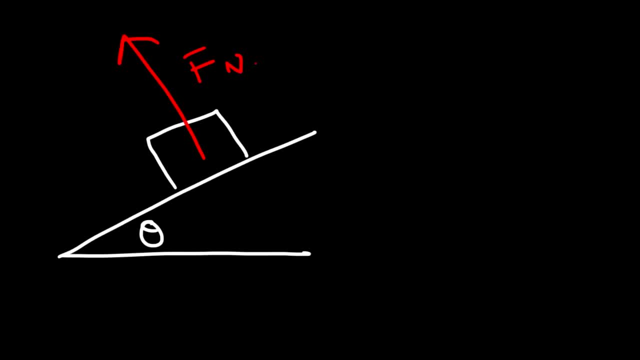 extend in this direction. It's always perpendicular to the surface And in this case the normal force will depend on the weight of the object and also the angle of the incline. It turns out that it's equal to the weight: mg times the cosine of that angle. 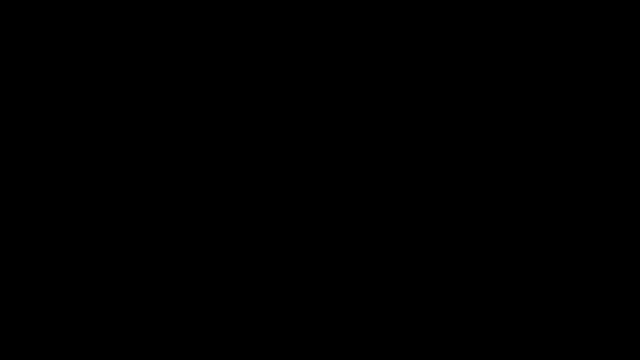 So, thestad, we don't have to keep studying it and try to calculate this. So far, we have covered the four forces: the applied force, the tension force, the normal force and the weight force, But what other forces are there that we need to learn in physics? 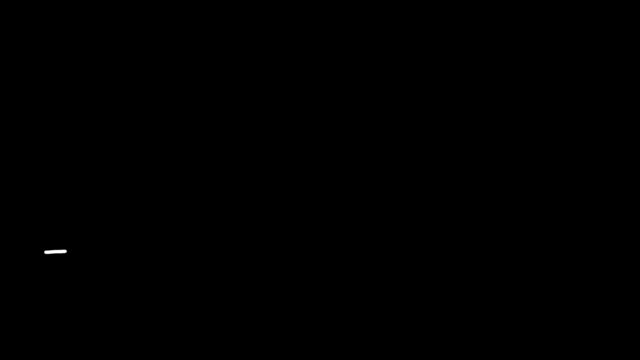 Now imagine a warm summer day and you're inside your home and you need to move this large box across a rough carpet, And so that's why this size and half, one and half مع. And so you apply a force to move the box, but it doesn't move. and you try to push it harder and it still doesn't move. 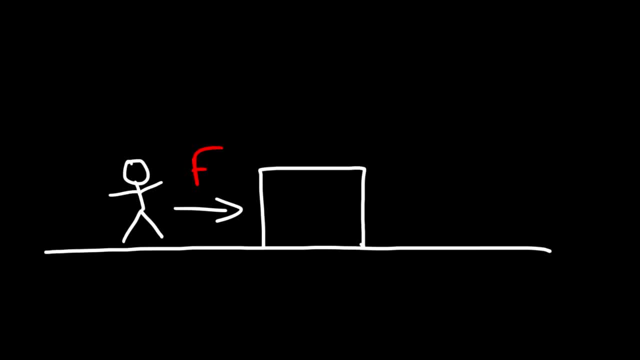 The question is why? What's preventing you from moving the box? Now, based on Newton's third law, for every action force there's an equal but opposite reaction force. So if you're applying a force to push this box and it doesn't move, there must be some other force that's preventing this box from moving. 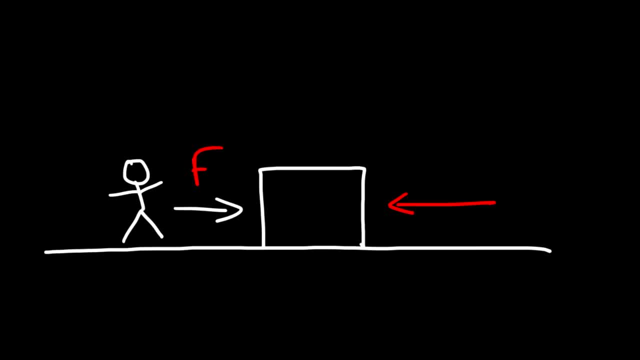 And in this case, this force is known as static friction. Static friction is present if the surface between the block and the ground, or in this case, the carpet, if they're not sliding past each other, and if there's Static friction is an applied force that doesn't exceed the maximum static frictional force. 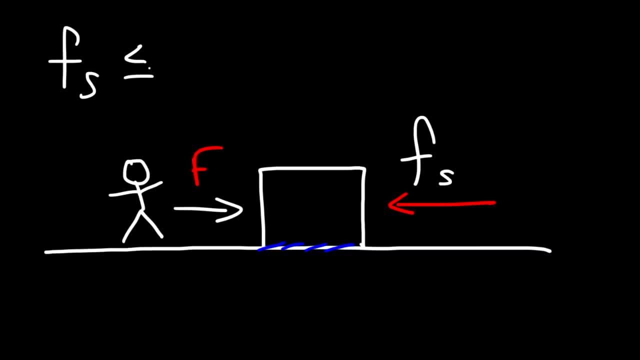 Static friction is basically an inequality. It's less than or equal to the coefficient of static friction, which is based on the interaction between these two surfaces, times the normal force of the object. Now static friction can be increased or decreased because the normal force can be increased. 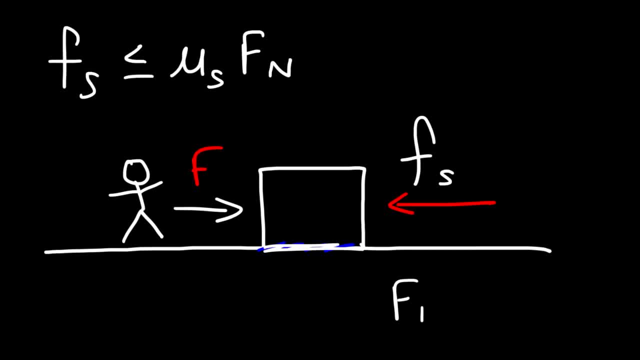 Now, earlier we said that the normal force is dependent on the weight of the object, and that's true, provided if there's no other vertical forces on this box. However, let's say, if I were to apply a downward force on this box, 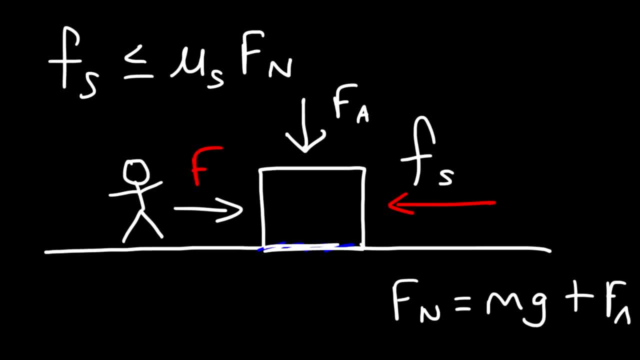 then the normal force will increase by that amount, And so, if I were to press down on that box, the static frictional force will increase. Now, at the same time, I can reduce the amount of static friction between the box and the carpet. 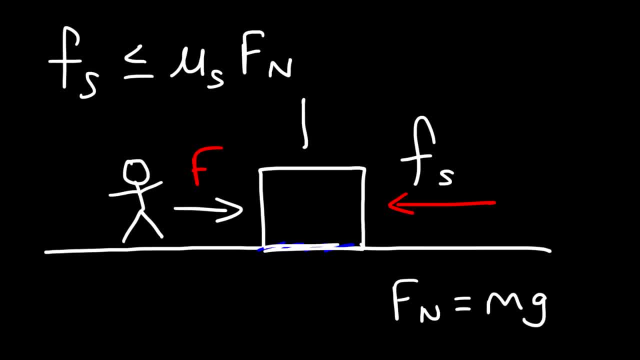 and that's by lifting the box off the ground, Or even if I don't lift it off, just by reducing the normal force. So let's say, if I had a rope and I pull the box upward with a rope, it doesn't have to leave the ground. 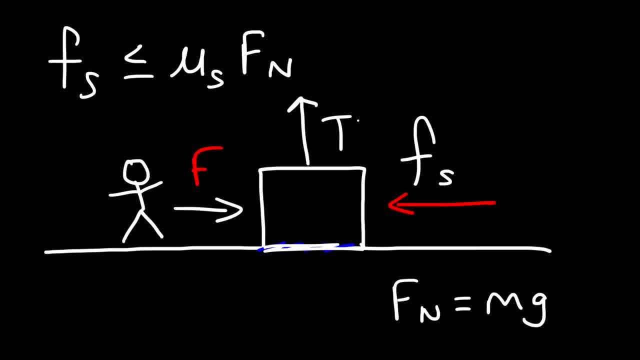 but basically relieve the stress that the block puts on the carpet. So if I lift it up with an upward force, the normal force will decrease by that tension force And thus, as a result, if the normal force decreases, the static frictional force will decrease as well. 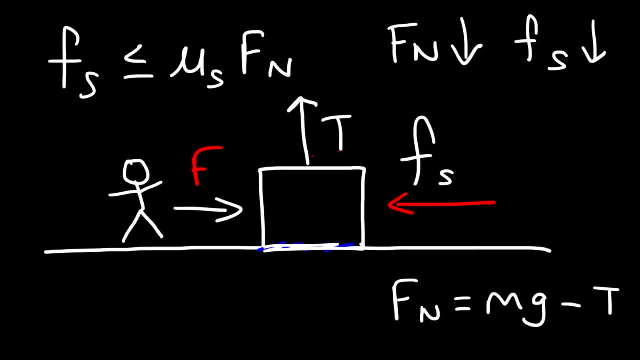 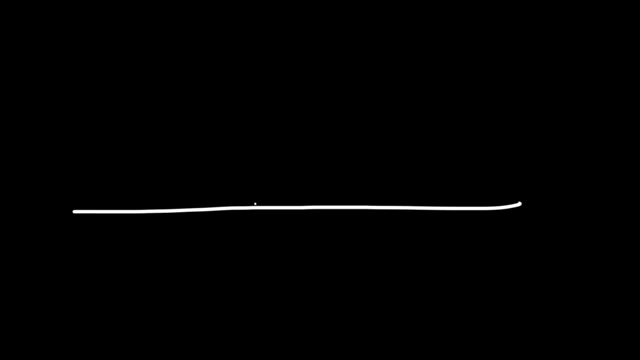 And so that's how you can reduce friction- is by lifting the object off the ground. Now, the next force that we're going to talk about is the kinetic frictional force. So if we go back to this example, and if this individual applies a force, 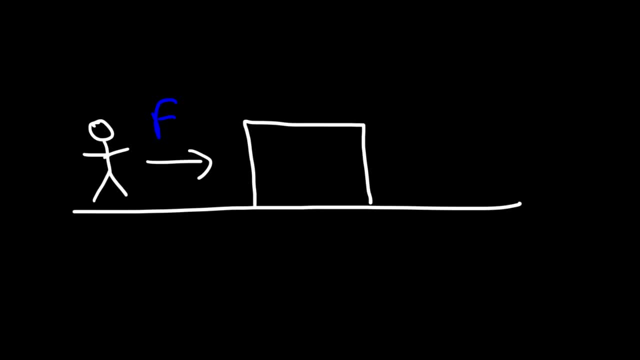 if the box doesn't move, as we said before, static friction is the reason that's preventing it from moving. Now, if the applied force exceeds the maximum static frictional force, then the box will begin to slide against the carpet. At that time, there's going to be another frictional force present. 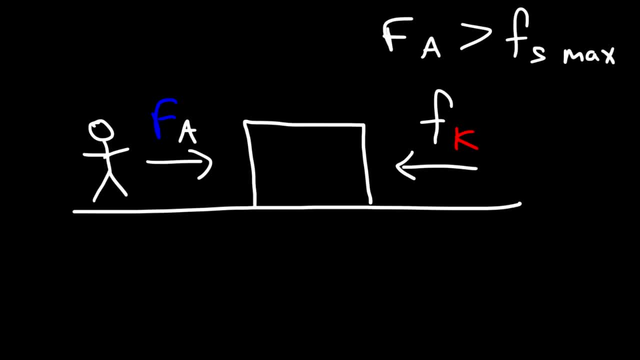 and it's called kinetic friction. Whenever you hear the word kinetic, it means motion, it means something is moving. Static means stationary, not moving. So static friction is present if these two surfaces are not sliding past each other, But if they are sliding past each other. 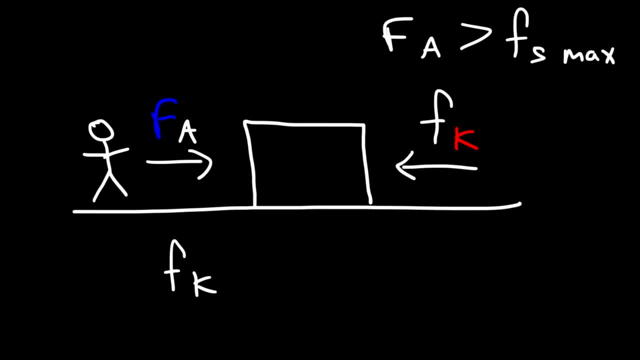 kinetic friction is present Now. the formula for kinetic friction is very similar to static friction. It's equal to mu k, the coefficient of kinetic friction times the normal force, Whereas static friction is an inequality. So static friction will equal the applied force. 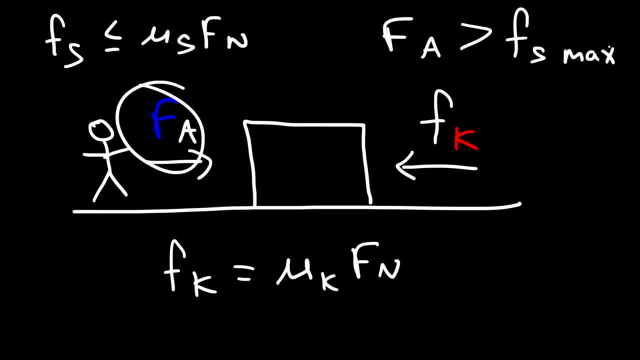 until the applied force exceeds the maximum static frictional force. So let's say, if the maximum static frictional force was 100 Newtons- Let me put this here- I'm going to put max- If the applied force is 50, the static frictional force will be 50.. 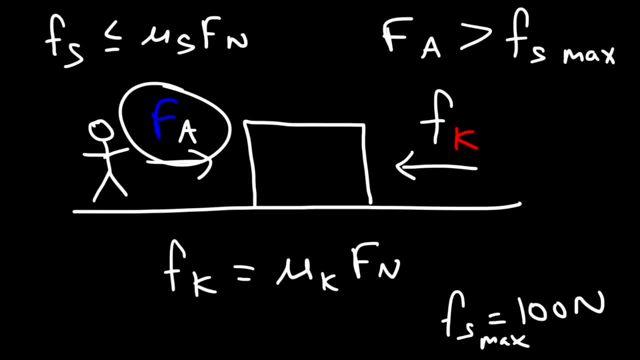 If the applied force is 80, the static frictional force will be 80.. If it's 100, this will be 100.. If the applied force is 120, then the box will begin to slide and you will no longer have static friction. 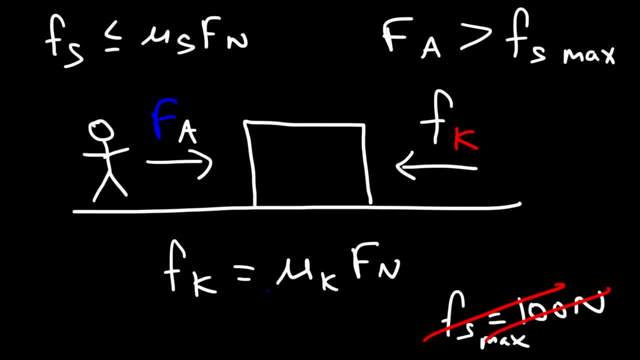 but now you have kinetic friction, which is equal to a fixed value. So if you increase the applied force, this value will not change. It's not an inequality, It's equal to a fixed number. Now the next type of force that we're going to talk about. 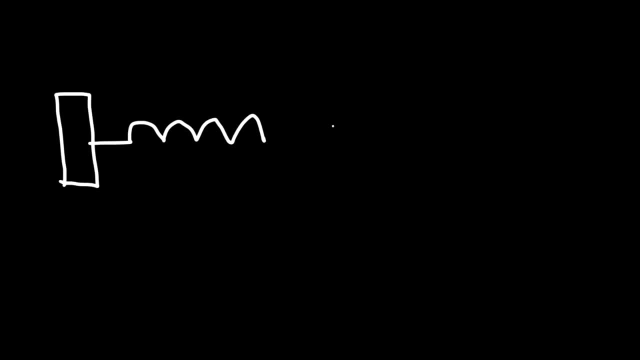 has to do with springs. So if you have a spring- and let's say this is the natural length of the spring- if you apply a force to stretch the spring, you're going to feel a restoring force that wants to bring the spring back to equilibrium. 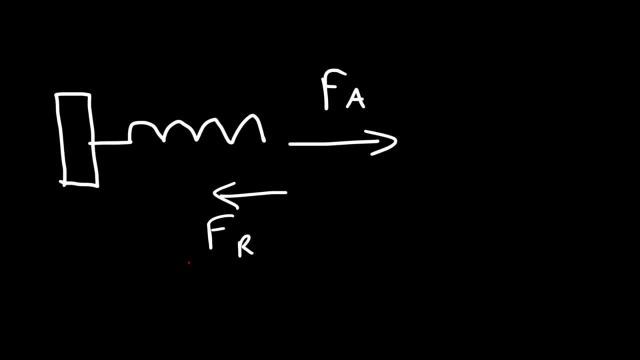 to its original position, And so this is another type of force that is present, And this is associated with something called Hooke's Law, which states that the restoring force is proportional to the spring constant k and x, where x is the difference between 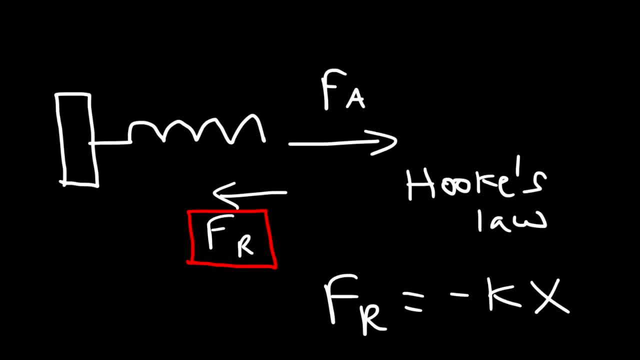 the original position and the new position. Now, k could be a value like 100 Newtons per meter, So that's the spring constant. That means that it requires 100 Newtons of force to stretch the spring by 1 meter or to compress it by 1 meter. 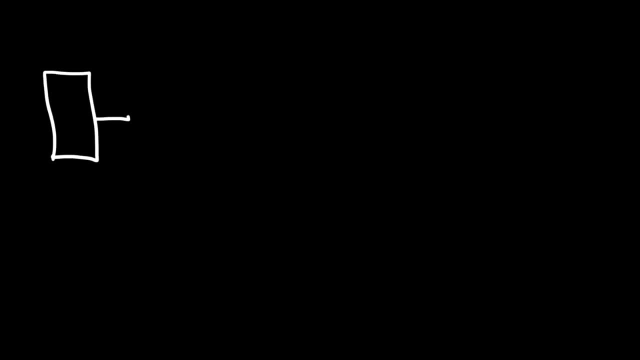 So let's say this is the original spring and let's say k is still 100 Newtons per meter And let's say I stretch the spring by 0.1 meters. So that is my x value. That is the difference in distance. 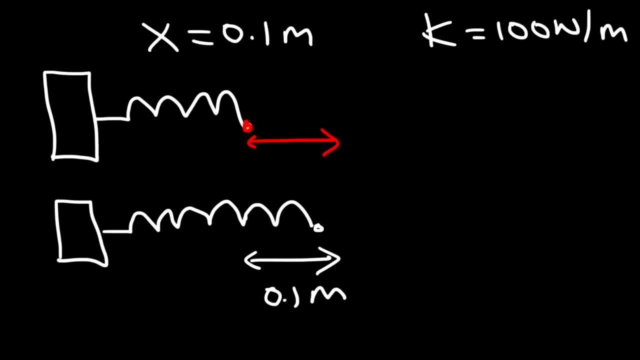 between the original point, where it's naturally located at, and the new point. So basically, x is the amount that I stretch or compress the spring from its natural length. Now, in order to do this, I need to apply a force that's equal to the restoring force. 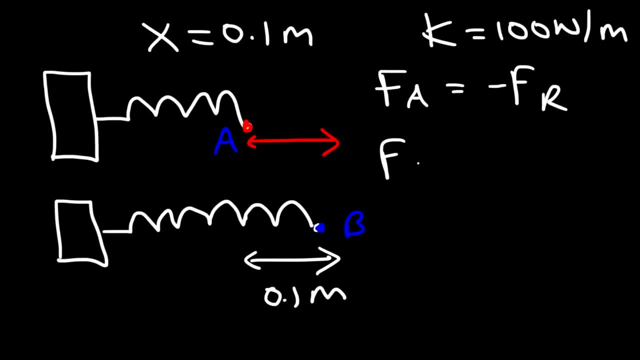 but opposite in direction. So the applied force will be k times x, So it's 100 Newtons per meter times 0.1 meters. So basically I need to apply a force of 10 Newtons to get the job done. 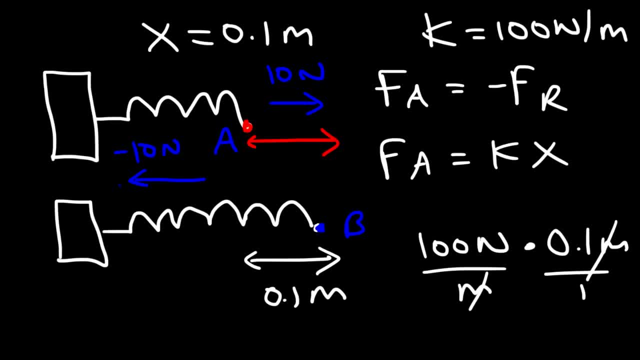 Now there's going to be a restoring force of negative 10 Newtons. The reason why it's negative is because it's going in the opposite direction, And so that's why, in this equation, we have a negative sign when dealing with the restoring force. 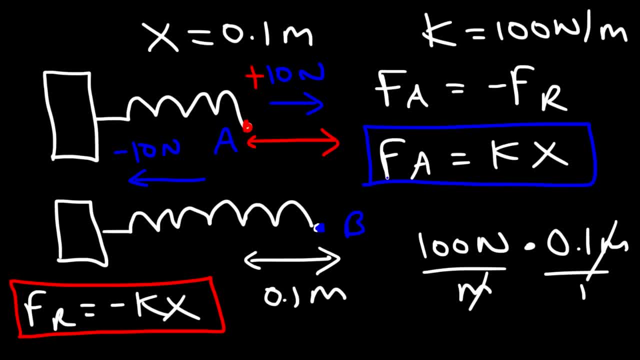 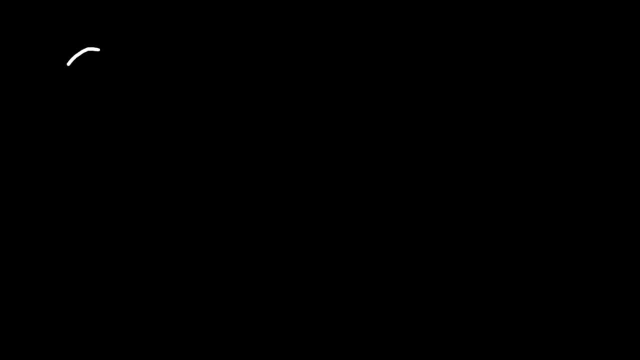 But the applied force will have a positive sign because, based on the way it's drawn, the applied force is directed in the positive x direction. Now, what happens to an object when the velocity of the object and the force that's acting on the object 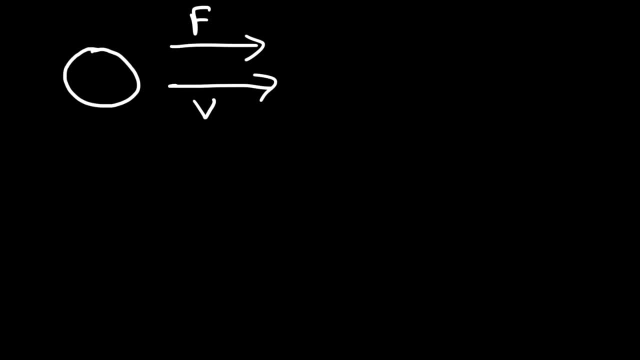 are in the same direction, What's going to happen to the object? Now compare that. let's say, if the object is moving to the right, but if there's a force that's acting on it, but towards the left In the first case. 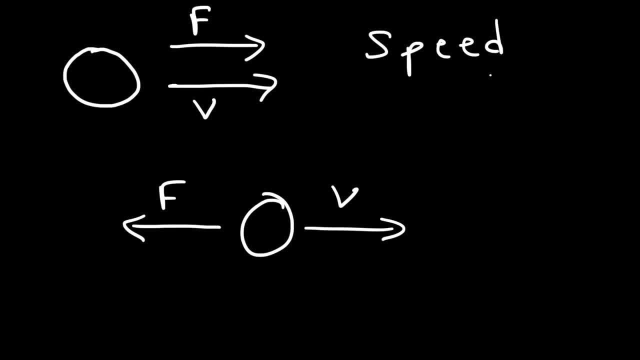 when the force and velocity vectors are in the same direction, the object is going to speed up. When force and velocity, when they're opposite to each other, the object is going to slow down. But now what happens if the force vector is perpendicular to the velocity vector? 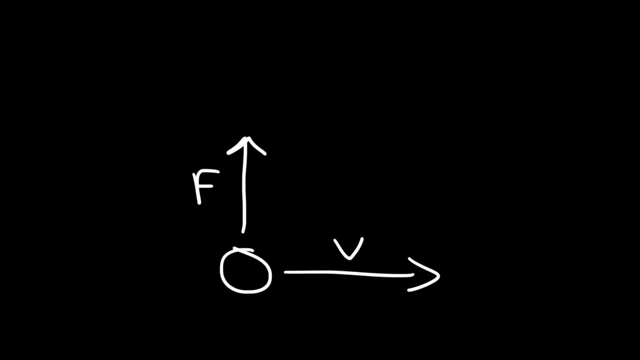 Will it speed up or slow down? In this case, the force has no effect on the speed of the object. However, it can affect the direction of the object. So in this case the object will turn And a force that causes an object. 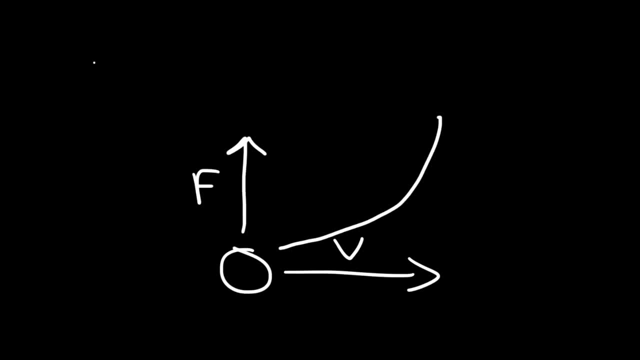 to turn in a circle is known as a centripetal force. Now, the centripetal force is not an actual force itself, but it's created or provided by other types of forces. Now imagine if you have a rope and a ball attached to the rope. 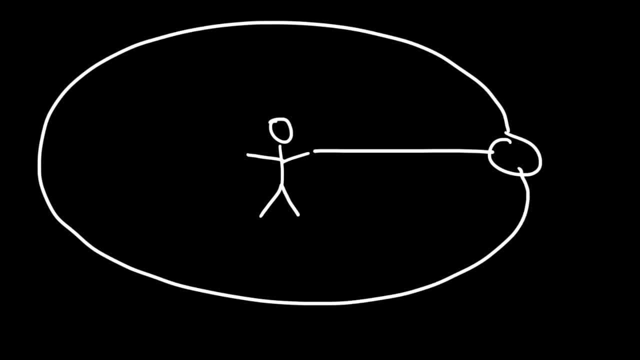 and you decide to swing it in a circle. What provides the centripetal force in this case? Now, at this point, the object is moving here in a positive y direction. However, there is a force called the centripetal force that is directed towards. 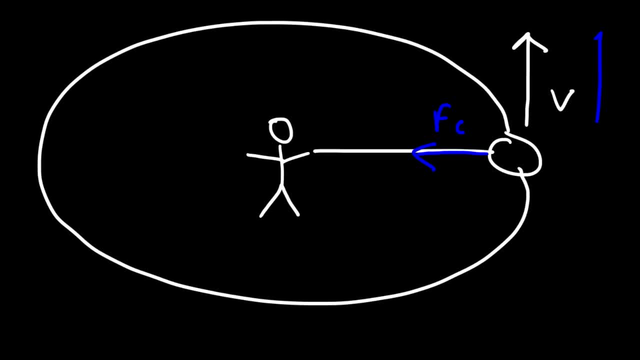 the center of the circle, And so the object will not go in this direction, but rather it's going to turn in the direction of the centripetal force. Now, once the object reaches this point, it's moving towards the negative x direction. 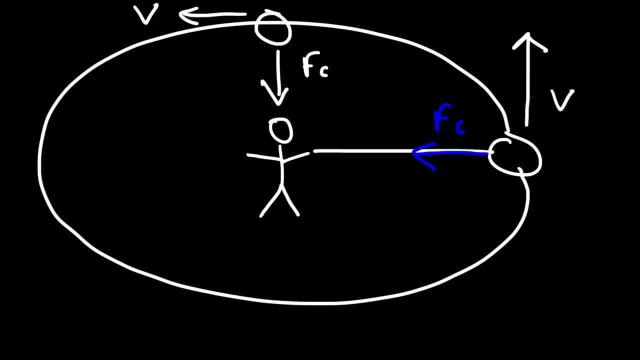 but the rope is going to be over here, and so the centripetal force is still pulling it towards the center, And so, once again, the object is going to turn, And so this process will be repeated. So when the object is on the left side. 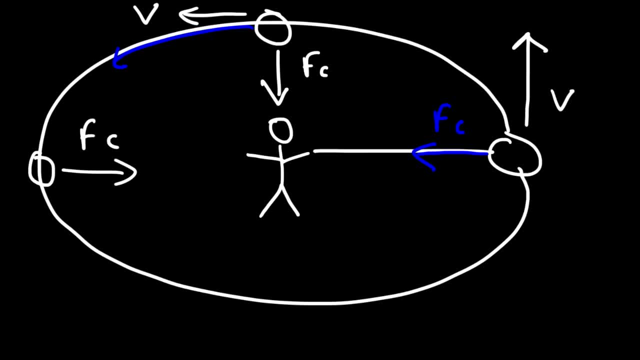 the centripetal force will be directed towards the right or towards the center, and the velocity vector will now be going down, And so the centripetal force is always directed towards the center of the circle, because it keeps the object moving in a circle. 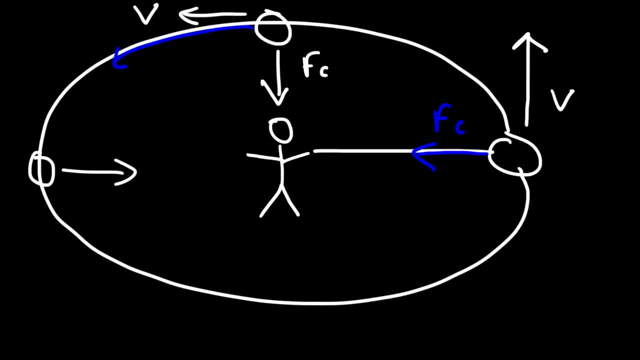 But, as we said before, the centripetal force is not in itself a force. It's always created by another force. So what is the force that provides the centripetal force in this example? Now here's a hint. What is the force that always act? 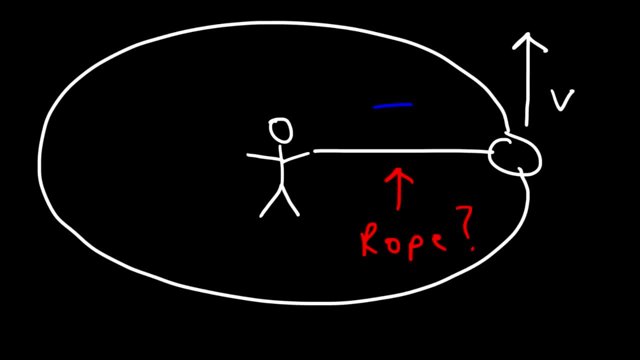 through a rope, There's always a tension force acting through a rope, So in this example, tension provides the centripetal force. Now I want to go over two different categories of forces. So you have contact forces and you have long-range forces. 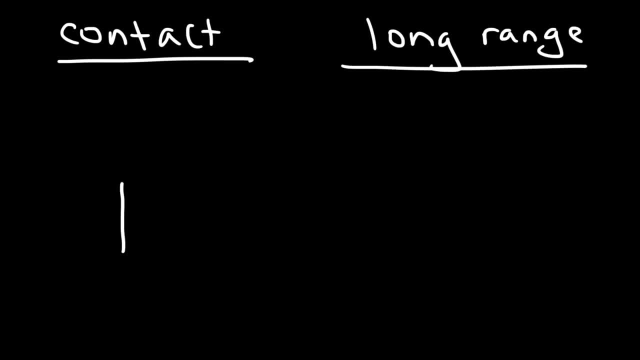 So we covered some examples of contact forces. In the beginning we talked about a person applying a force to push a box, And so that applied force is a contact force because it can only exist when the person is in contact with the box. 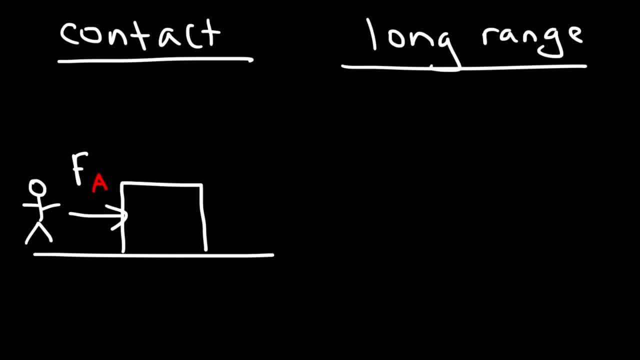 Now, a long-range force doesn't require a contact to have an effect. For instance, gravity is a long-range force. So let's say: this is the ground, which is the surface of the Earth, and there's a ball. Gravity will cause. 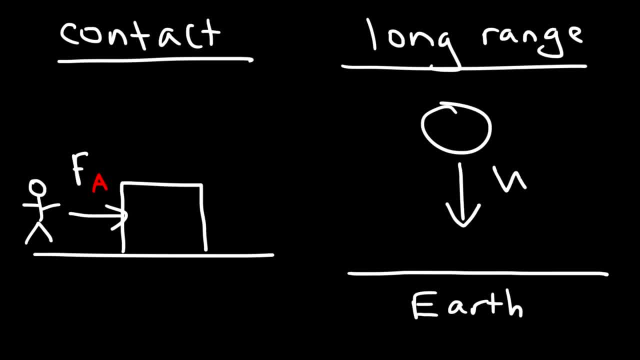 the ball to fall, And so gravity exerts a force on the ball, which is known as the weight force, And the ball doesn't have to be in contact with the Earth. It could be in the air, and yet the Earth can still exert. 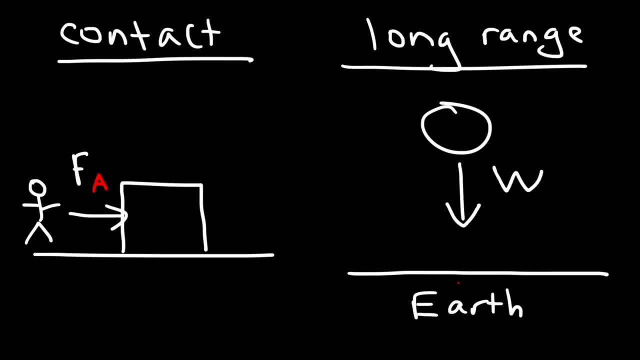 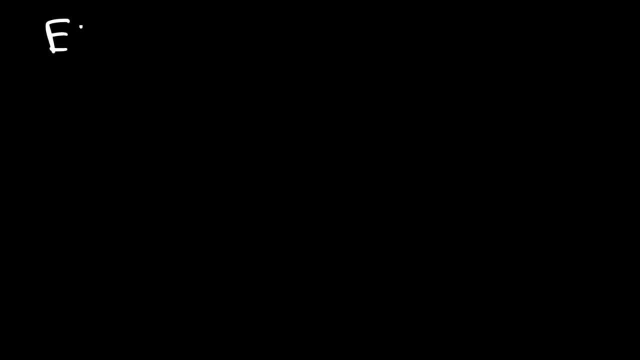 force on a ball. So gravity is an example of a long-range force. Another example of a long-range force is the electric force. So let's say, if we have a positive charge next to a negative charge, These two will fill a force of attraction. 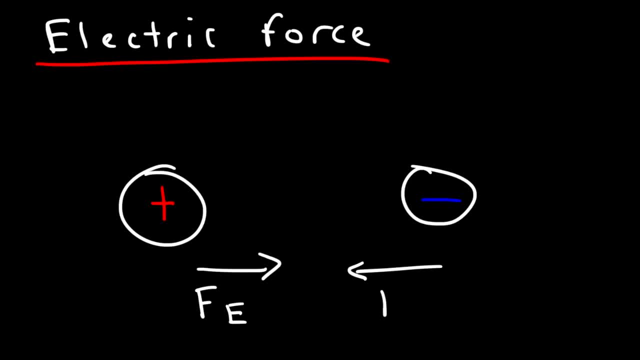 And so they fill an electric force that accelerates them toward each other, And they don't have to be in contact to fill this force or to be affected by it, And so the electric force is a long-range force. Now, the electric force. 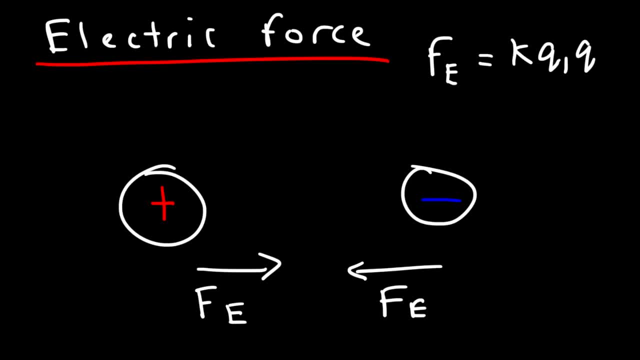 is equal to k times q1 times q2 over r squared. Now, k is a constant, It's equal to 9 times 10 to the 9.. And uh, q1 and q2, they represent the charge of these two particles. 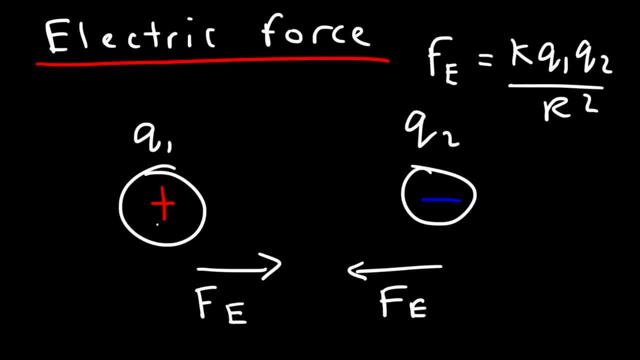 or two objects And the units for that is coulombs, And r is the distance between them. Now there's two ways in which you can increase the electric force between these two charged particles. One, by increasing the magnitude of the charge. 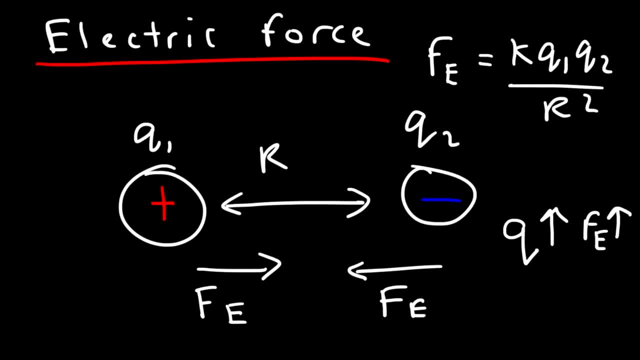 on each of them, That will increase the electric force between them. Or if you bring the charges closer together, the force of attraction that they will fill will be greater. So if you decrease r the electric field, I mean not the electric field, but 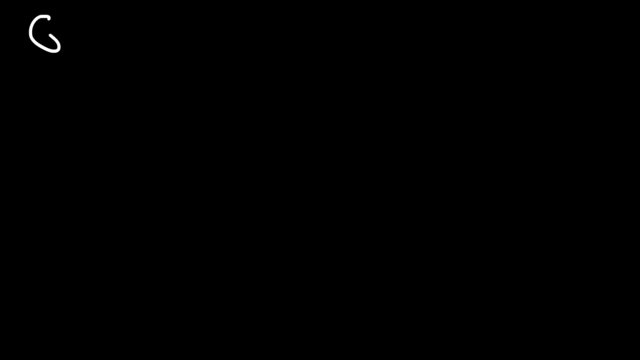 the electric force will increase in magnitude. Now let's go back and talk about gravity. So we saw that there is an electric force between two objects that have a charge. If they have opposite charges, the two objects will be attracted to each other. 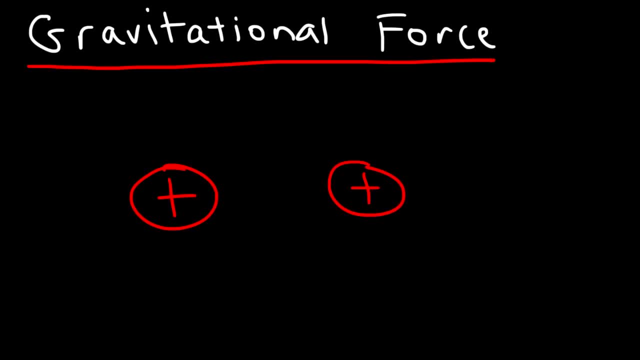 But between two like charges they will be repelled. So the electric force can be a force of attraction or a force of repulsion. The gravitational force is a force of attraction And it exists between two objects with mass. Say, if we have the sun, 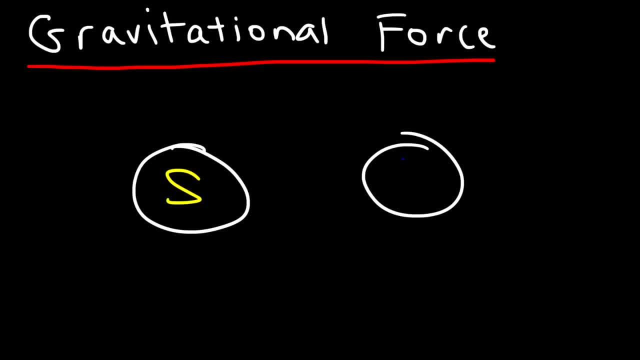 let me use a different color for that- and the earth. So between two objects with a large amount of matter there's going to be a force of attraction known as gravity, And so gravity brings matter together, And the formula for it is: F is equal to. 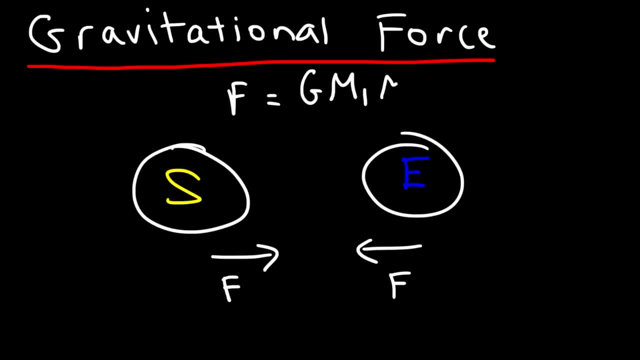 G, the universal gravitation, constant times m1 times m2 over r squared, Where m1 and m2 are the masses of these two objects. So if you increase the mass of an object, the gravitational force will increase, And if you decrease the distance, 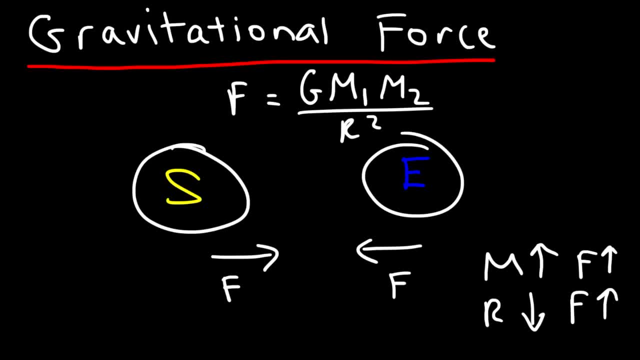 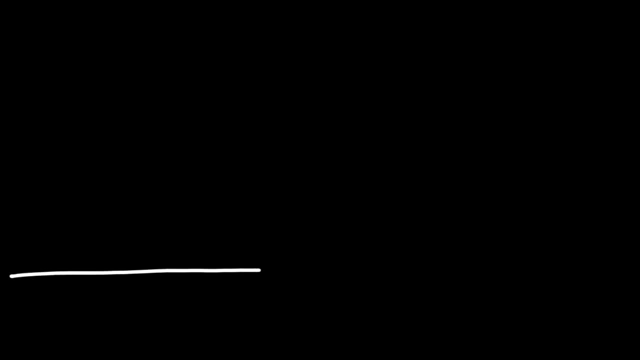 between them, the gravitational force will increase as well, And so the more massive the sun is, the greater the gravitational force that it will have on the earth, So its pull on the earth will be stronger. Now let's say this is the. 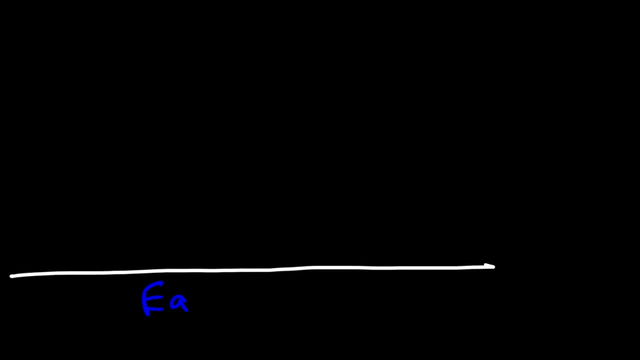 surface of the ground which, as we said before, is the surface of the earth. And let's go back to the example where we had the ball in the air. Now the earth will pull the ball down, It's going to exert a gravitational 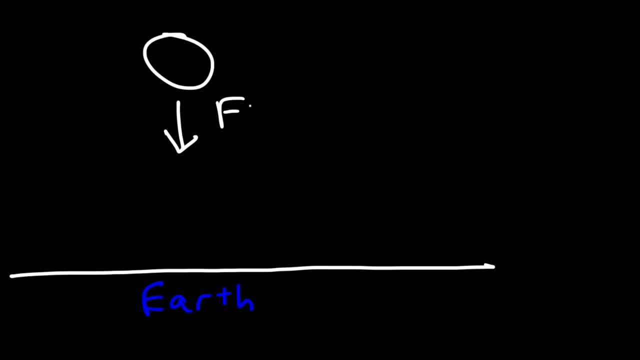 force on the ball which will accelerate it in the negative y direction. Now, based on the last example, where we saw that the earth and the sun, they both exerted a gravitational force on the earth And that means that the ball exerts. 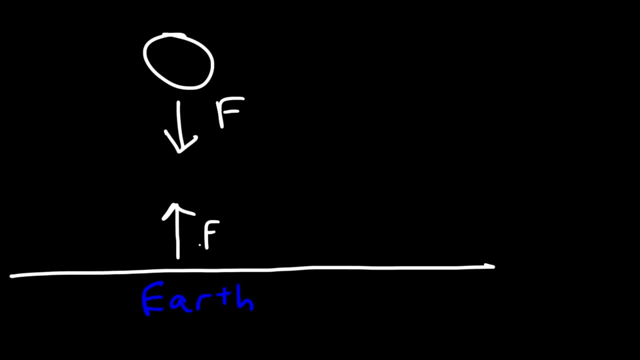 a gravitational force on the earth, causing the earth to move towards the ball. Now, granted, the earth is much more massive than the ball, so it's not going to move by much, It's going to be negligible, But there is a force that 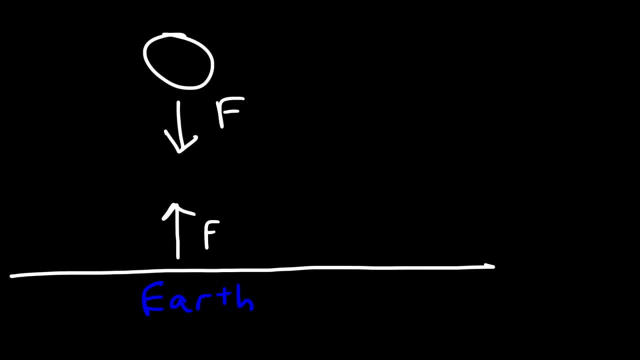 pushes the earth towards the ball, But because the mass of the ball is so little, it's insignificant, But yet the ball doesn't fall towards the earth. It's falling in that direction. So if the ball is falling towards the earth, 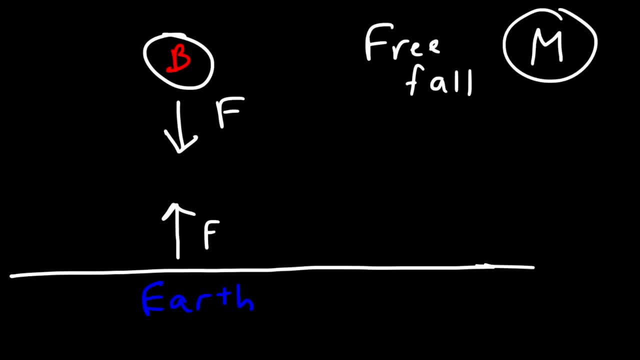 what about the moon? Can the same be said of that? Why doesn't the moon just fall to the earth? How does it remain in orbit? Because this ball, if you put it in the air, it's just going to fall towards the earth. 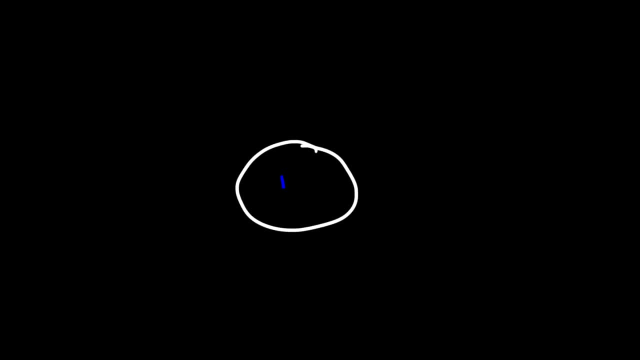 So let's draw another picture. So let's say: this is the earth and this is the ball. So if we put the ball in outer space, it's simply going to drop to the earth. It's going to be in free fall. 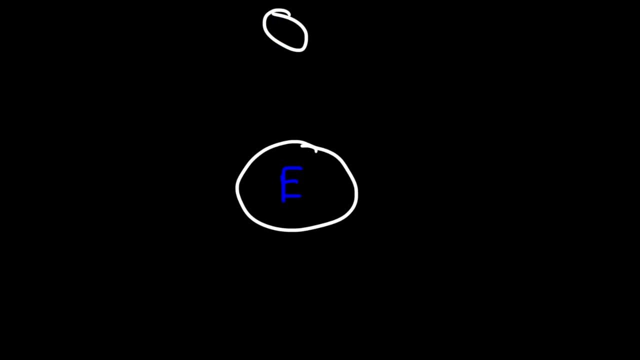 It's going to crash and that's it. But the moon, if we put it here, it too, is in free fall towards the earth, but it doesn't crash into the earth, which is a very good thing, because that would be catastrophic. 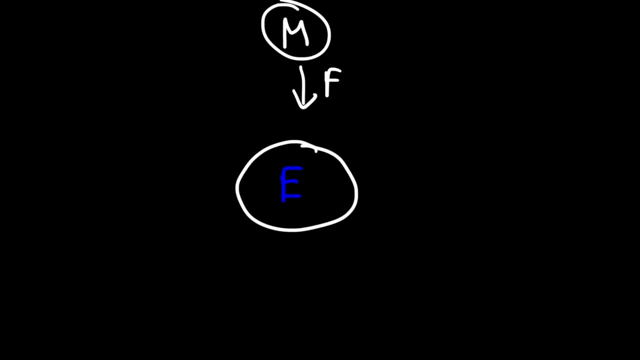 But why doesn't the moon not fall towards the earth like the ball? And the answer is velocity. The moon is moving in this direction at this instant in time And, as we saw in a previous example, whenever the force and velocity vectors are perpendicular, 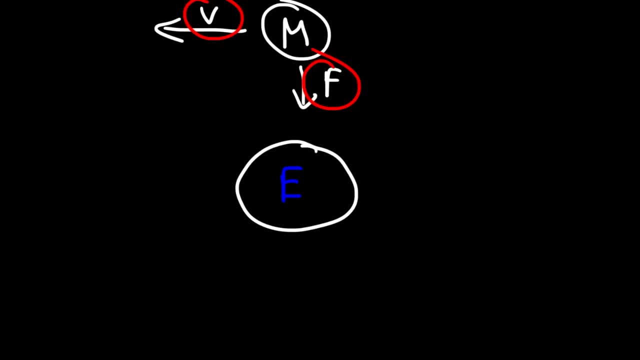 if they're 90 degrees apart from each other, the object is going to turn, and so the moon turns in a circular path. And that's how the moon can remain in orbit. It's due to the balance of the gravitational force and the velocity of the moon. 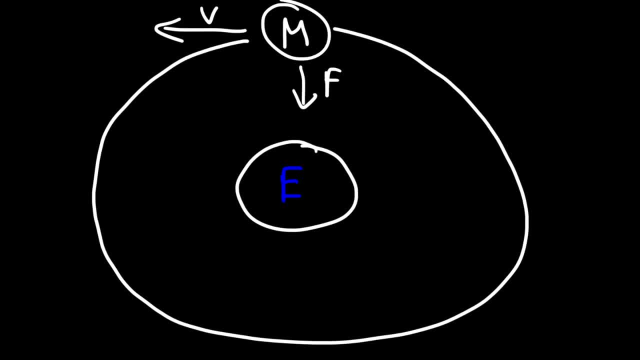 Now, what other type of force do we have here? Because there exists a certain type of force. any time, that force is pointed towards the center of a circle, If you recall, this is the centripetal force. Now, the centripetal force is always caused by another. 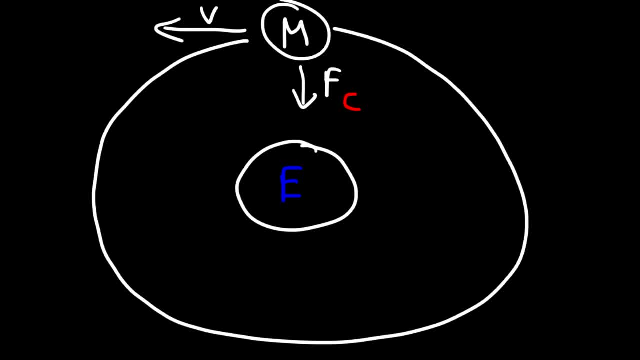 force. So in this particular example between the earth and the moon, gravity provides the centripetal force for the moon. Gravity keeps the moon in orbit around the earth. If gravity wasn't present, the moon would fly off towards outer space And 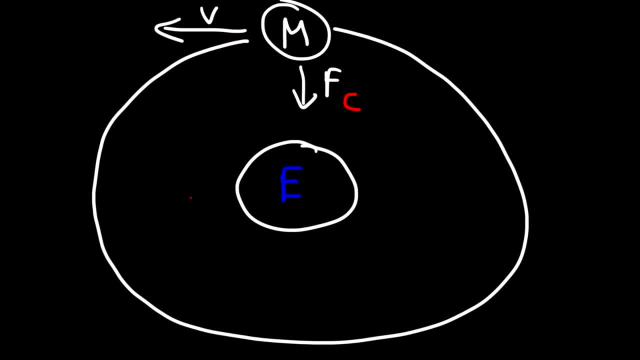 if the moon didn't have this velocity, it would free fall towards the earth crashing into it. So, due to the balance of the moon's speed and the gravity between the earth and the moon, it remains in orbit. Now the next type of force that you'll hear about. 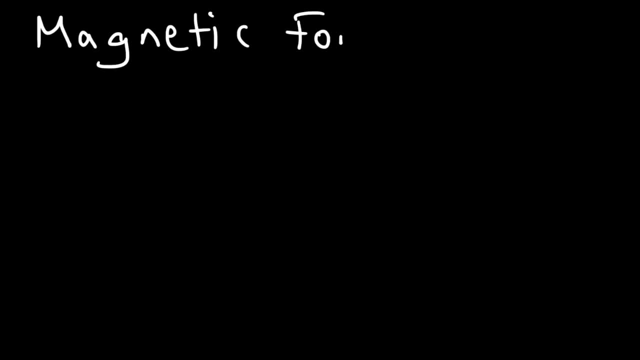 in a typical physics course is the magnetic force. Now, I'm sure you're familiar with magnetism. At some point in your life you played with magnets and you know that the north pole of one magnet is attracted to the south pole of another. 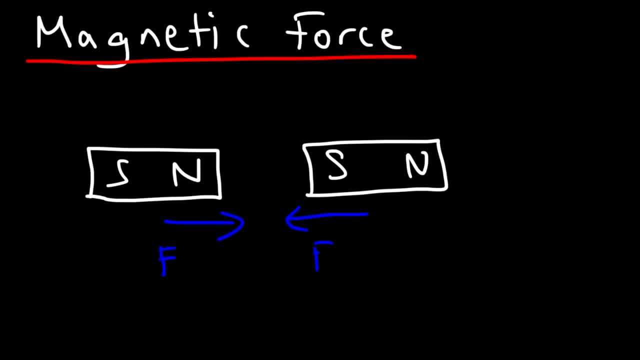 And so these two magnets will feel a force of attraction. Likewise, if you have two bar magnets with the north pole facing each other, these two will feel a force of repulsion, And so that's one example of a magnetic force that you've seen. 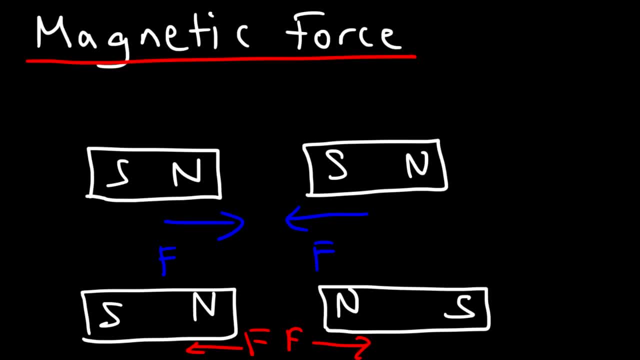 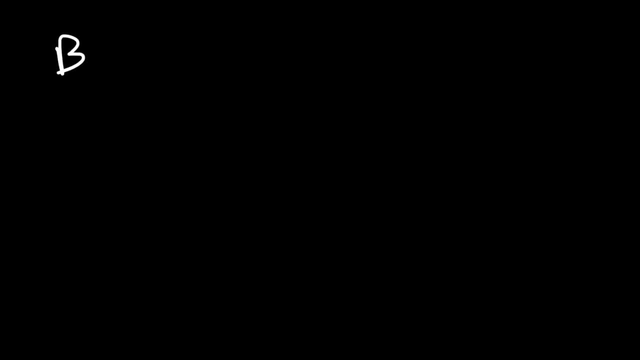 But in a typical physics course you're going to see how magnetism relates to charges. And let's say we have a magnetic field represented by the symbol B and it's directed into the page. So that's what that X means In physics, if you see this symbol. 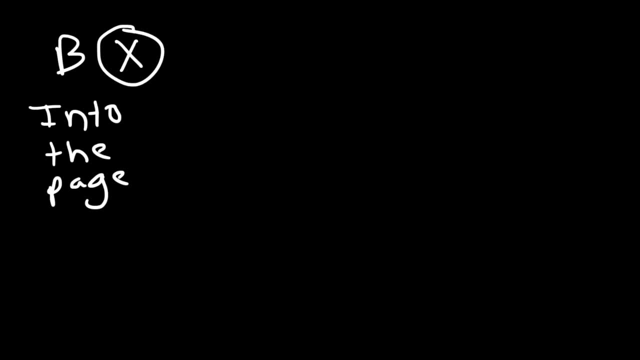 that means that the magnetic field is coming out of the page. So in a three dimensional system we have the Z axis, the Y axis and the X axis. Now into the page means that the magnetic field is going in the negative Z direction, Out of the 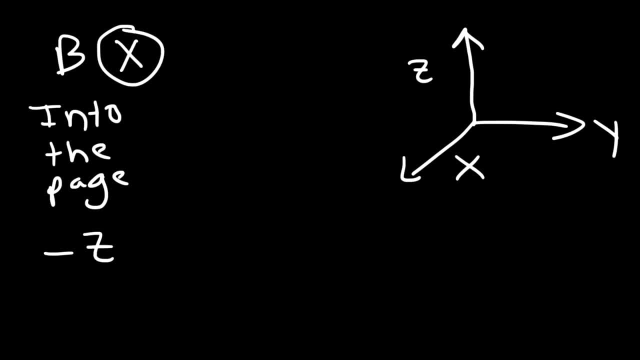 page means that it's going in a positive Z direction. So just keep that in mind. Now let's say, if we have a proton and this proton is moving to the right Now using the right hand rule, which I won't go into too much detail in this video, 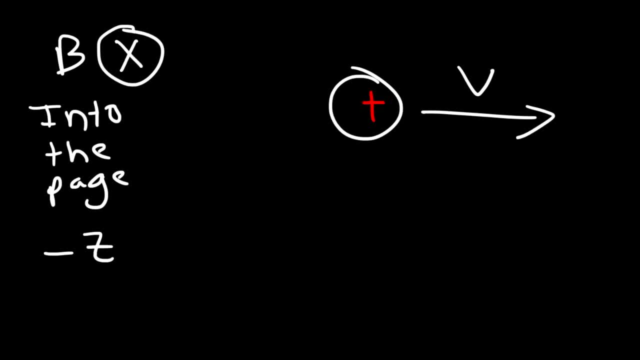 but you can look up another video I have on YouTube that explains it. Just type in right hand rule- magnetic fields and it should come up. So if we have a proton moving in a positive X direction and a magnetic field going into the page, 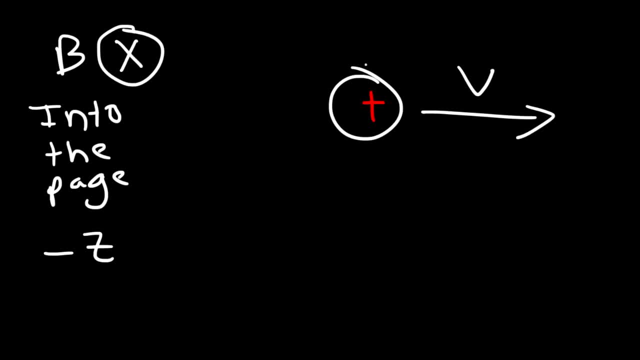 in a negative Z direction. using the right hand rule, the magnetic field will exert a magnetic force, FB- in the positive Y direction, Now an electron. if it's moving towards the right, it will feel a magnetic force in the opposite direction. 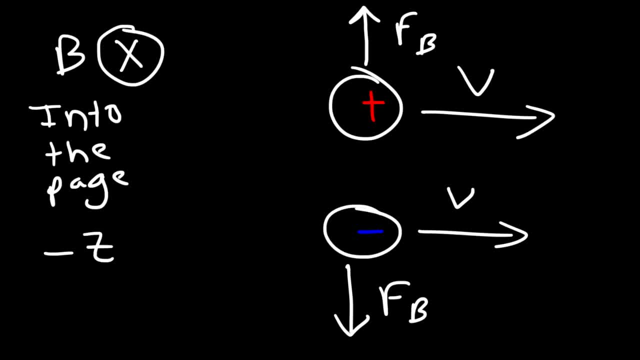 to a proton that is in the negative Y direction. So what you need to understand is this: If you have a charged particle that is moving in a magnetic field, the magnetic field will exert a force, a magnetic force, on that charged particle. If it's not, 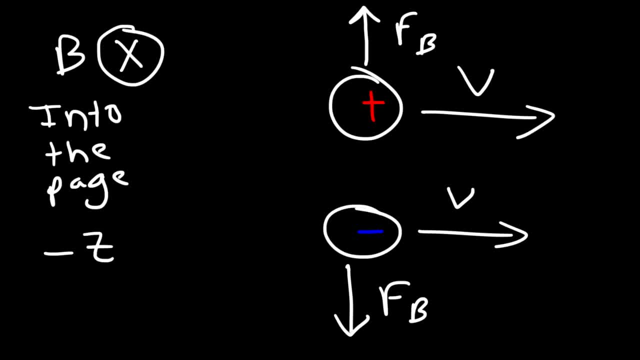 moving, it will not exert a magnetic force. And the magnetic field, the velocity and the magnetic force, they're all perpendicular to each other. One is in the X direction, the other is in the Y and the third one is in the Z direction. 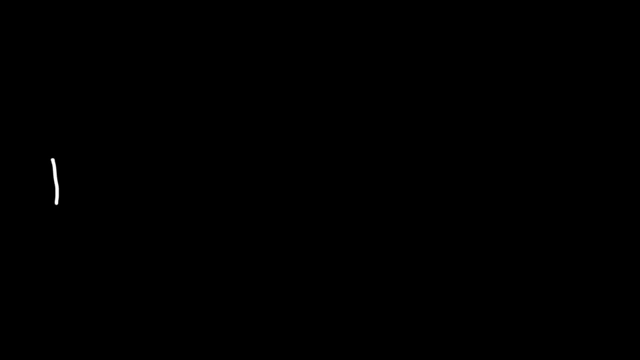 So they always are perpendicular to each other And you can create a magnetic field just by using a bar magnet. So let's say: this is the North Pole and this is the South Pole, So the magnetic field extends out from the North Pole. 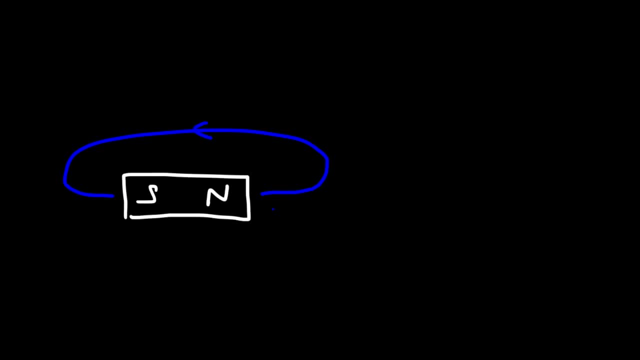 and it flows towards the South Pole. So if you have another magnet, this will also have its own magnetic field. So if we focus on the magnetic field between these two magnets in this region, the magnetic field emanating from the magnet on the left- 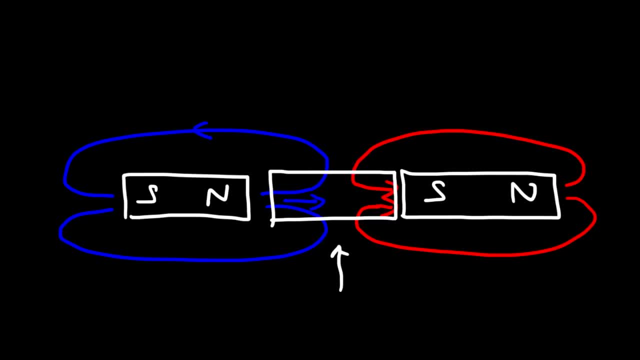 is going in the positive X direction, And the magnetic field entering the second magnet on the right is also going in the positive X direction, And so it has an additive effect. So the magnetic field in this region is very strong. Now, if we were to place 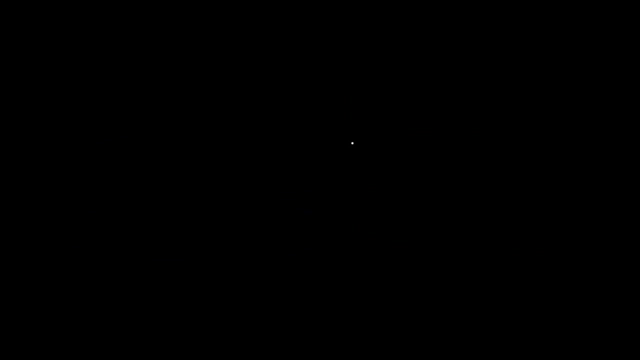 let's say, a moving charge in that region. so we have the magnetic field going in the positive X direction and let's say there's a proton in that region And that proton is moving in the positive Y direction and that means that it's going to fill. 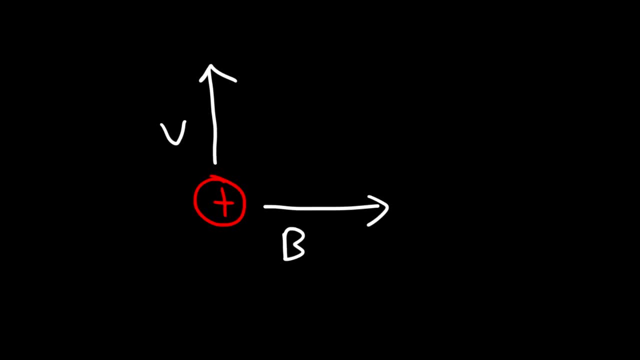 a magnetic force in the Z direction. So, using the right hand rule, let me use it real quick. this is going to be into the page And so we can represent it with this symbol. So the magnetic force is going in the negative Z direction. 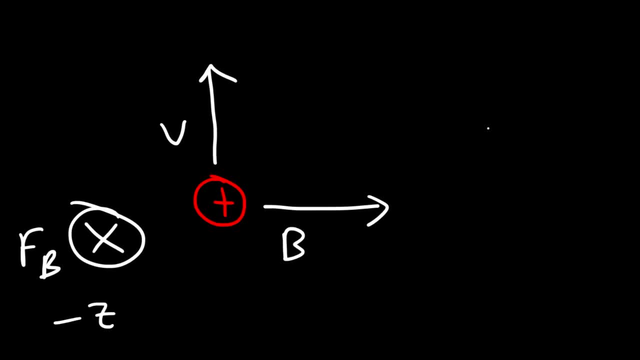 And if we were to draw a three-dimensional coordinate system? so this is the positive X direction, this is the Y direction and this is the X direction. The magnetic field is going in the positive X direction, The proton, which I'm going to. 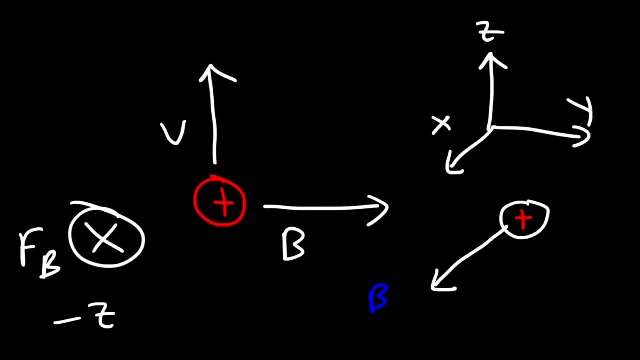 put in the center. it's moving in the positive Y direction and the magnetic force is being directed in the Z direction. So hopefully that three-dimensional coordinate system can give you a better visual of what's happening here. Now, going back to the first example, 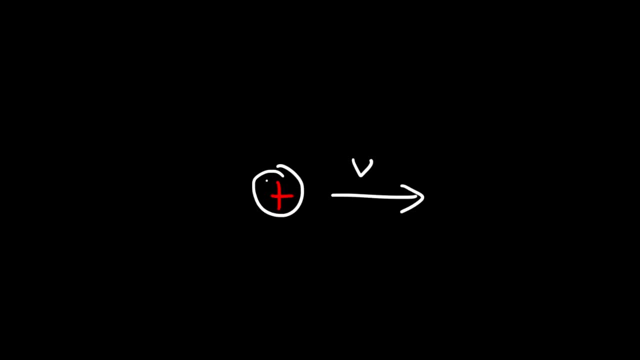 where we had the proton moving to the right and we had a magnetic field going into the page and we said that there was a magnetic force in the positive Y direction. So notice that the force and the velocity vectors are perpendicular. So in this case, 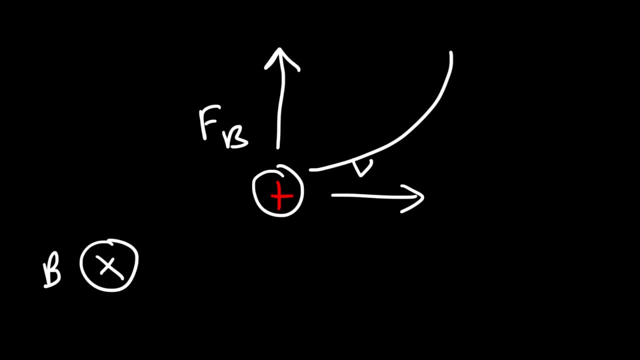 the object will turn. So whenever you have a moving charged particle in a magnetic field, it follows a circular path. The magnetic field becomes a centripetal force. It keeps the particle moving in a circle, And so let me redraw the proton here. 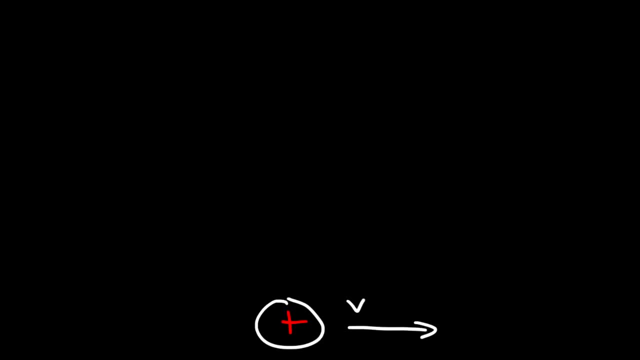 So if the proton is moving in this direction, there's a magnetic force that's going to be going in a positive Y direction, and so the proton is going to turn. It's going to follow a circular path. So when the proton is in, 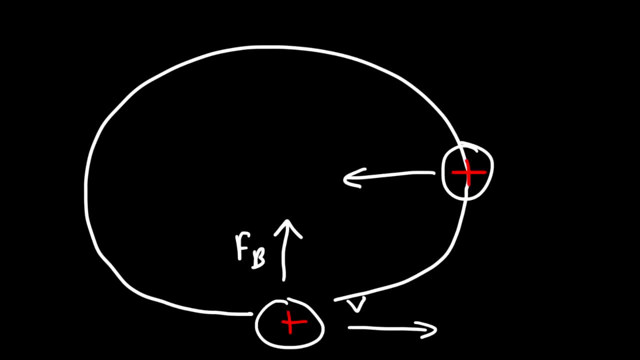 this region, the magnetic field will be directed towards the center and the proton is moving upward, And then, once it's at the top, its velocity vector will be directed to the negative X axis and the magnetic field will be directed towards the center. 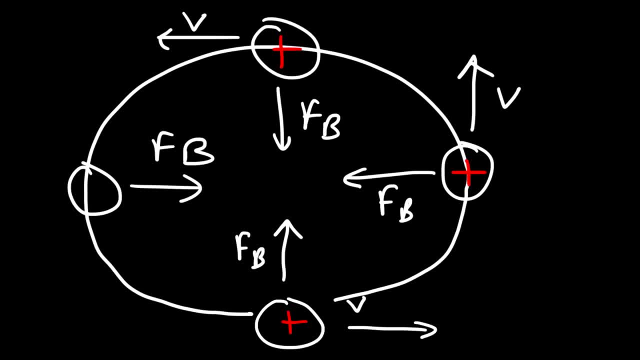 And so the magnetic force is acting in such a way to keep the proton moving in a circular path. So we saw three examples of other forces providing this centripetal force. We saw tension where, if you have a ball attached to a rope and if you swing it in a circle, 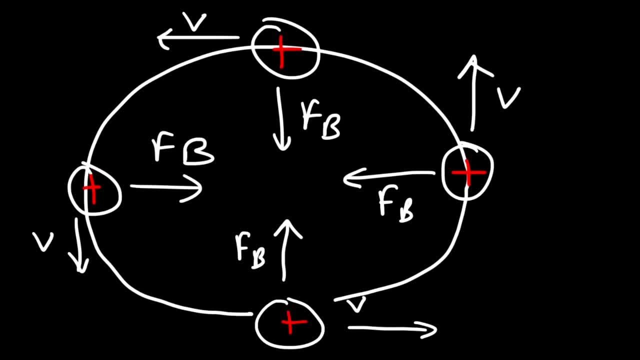 tension provides this centripetal force. In the second example we saw the situation between the Earth and the Moon, How the Moon was moving in a circle around the Earth and so gravity provided the centripetal force in that case And for this example, the magnetic force. 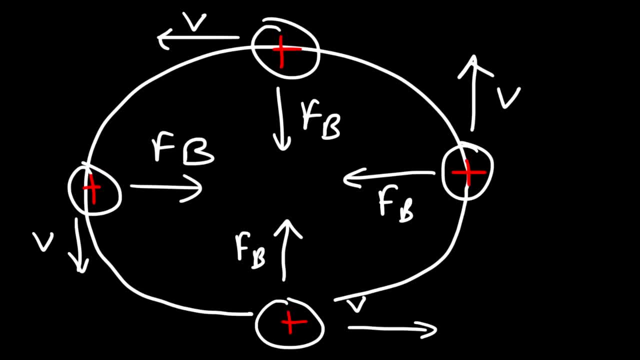 is keeping the proton moving in a circle. so the magnetic force provides the centripetal force. So make sure you understand that The centripetal force is not a force in itself, but it's generated by another force. It's any type of force.